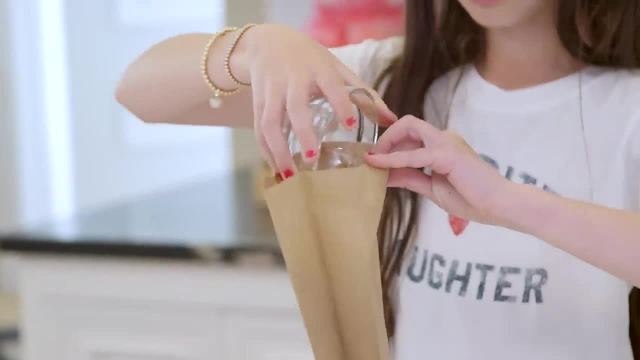 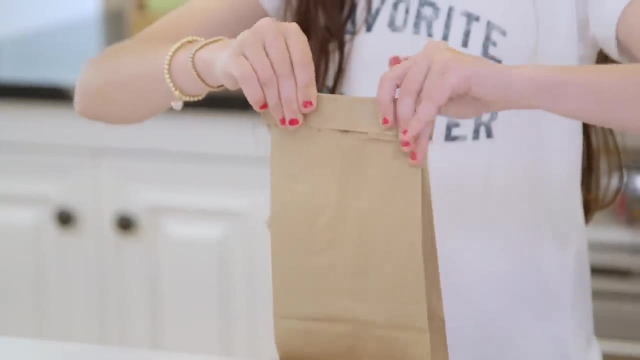 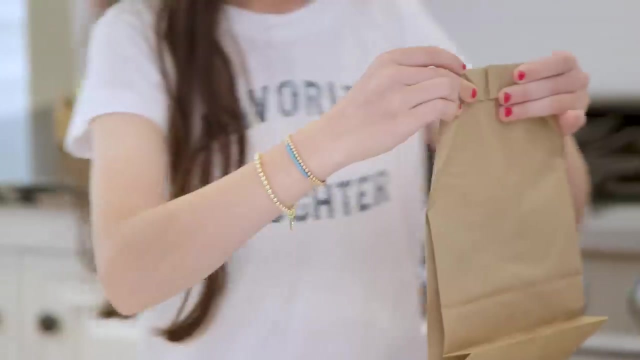 You're going to pour the kernels into the bag Makes a nice sound. Now you're going to fold it over like this. You're going to fold it like this and like this, And then you're going to stick it into your microwave. 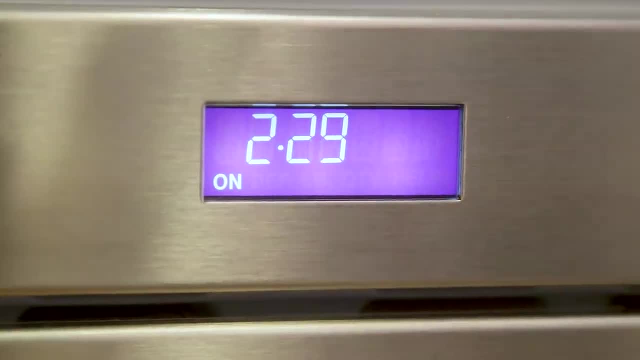 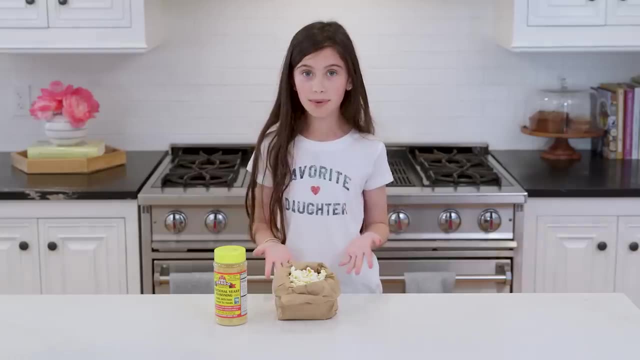 Lay your bag down flat and turn your microwave on for about two and a half minutes. You know it's done when the popping slows down. Popcorn is done. Popcorn is done. Popcorn is done, And in order to make it salty, you would have to put some oil on it, or butter, and then put the salt on. 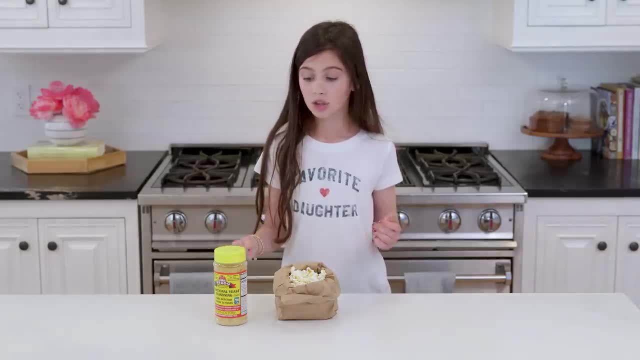 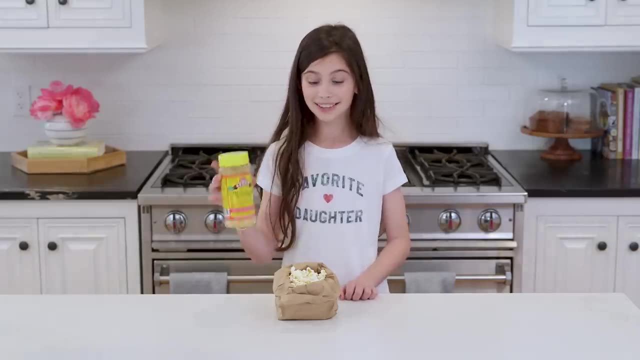 And that really doesn't pass the greasy fingerprint test. So you can also add nutritional yeast, which mom says is healthy and it makes it taste cheesy. But I'm just going to eat it plain. Really good. Now we're making Pop-Tarts. 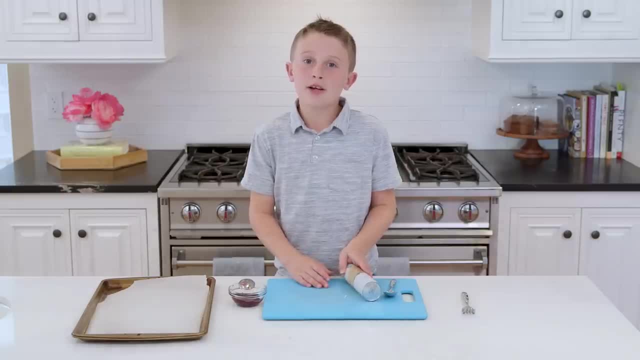 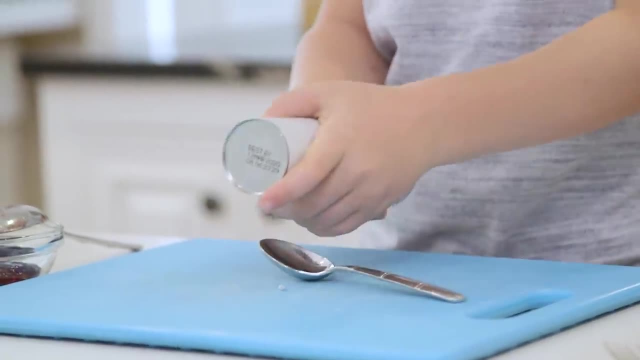 I love these because these are super easy to make, because we're using crescent rolls. Okay, so now I'm going to open my crescent roll. I'm good at this. I've had experience. I'm a pro. Okay, so we have two in here. 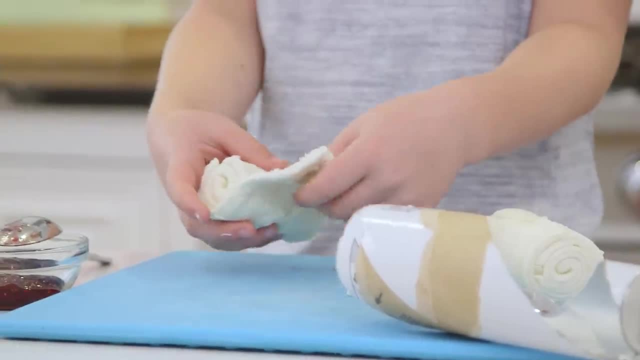 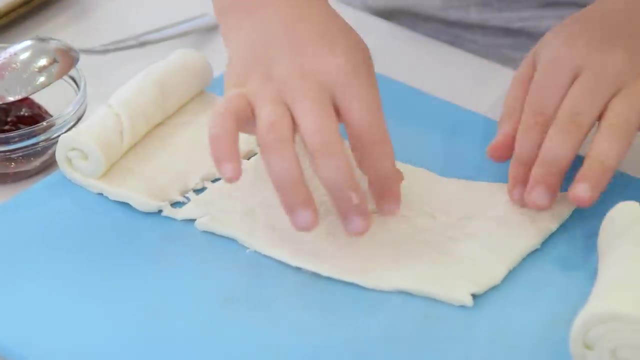 I'm going to take them out. The key is don't make them into triangles. So I'm unrolling them carefully, Not too careful. Yeah, I have a rectangle here, Not a triangle. There's two triangles, but I don't want a triangle. 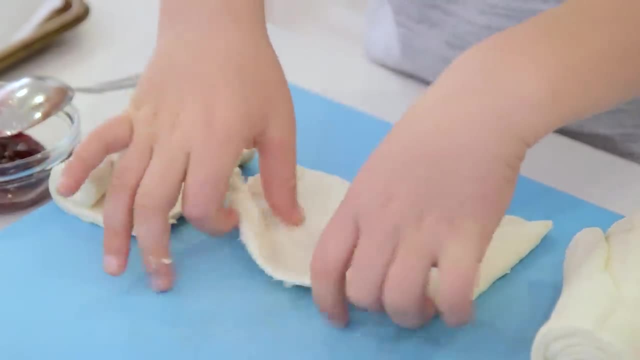 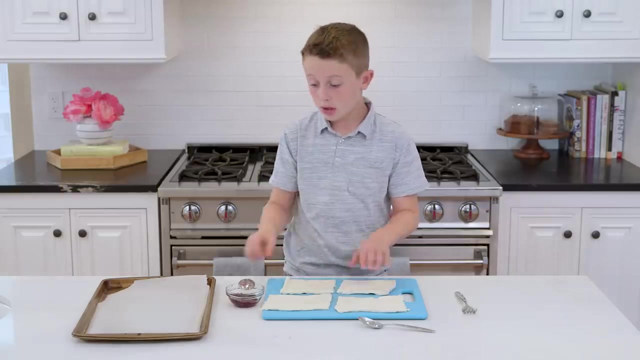 So I'm keeping those together and not separating them. I'm pinching the seam, Don't want any jam to leak through, So my base is ready. now I'm gonna use my jam. So I'm gonna scoop up a bit of jam and it's very important that you only put it in the 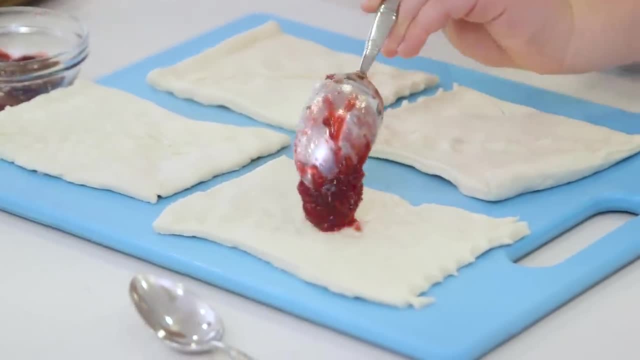 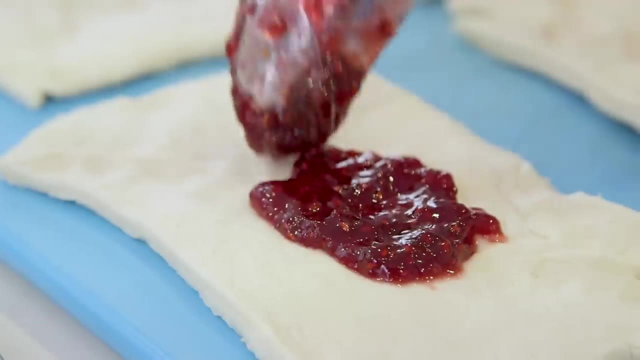 middle, not in the sides, because the sides are. these are gonna stick on top of each other. Got some jam and I'm putting it in the middle and I'm gonna use the back of my spoon to spread it out. Next up is to take the other. 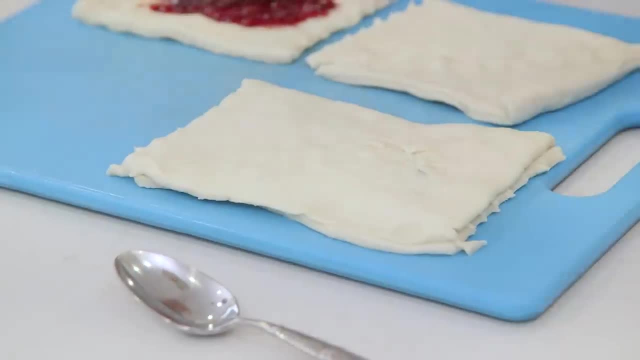 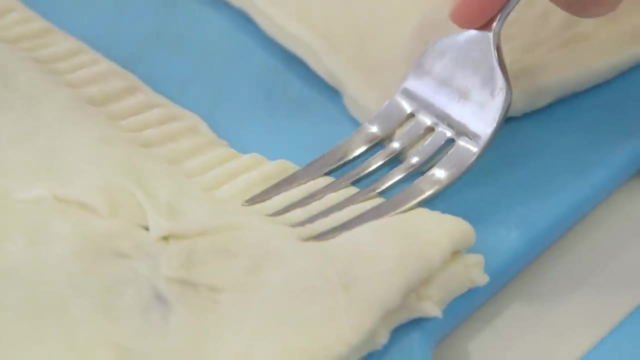 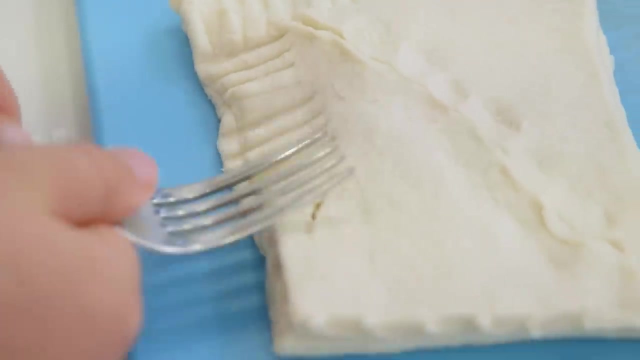 rectangle, place it right on top. I'm gonna take a fork, I'm gonna press it down just enough to make them stick together. still make it look pretty. These are looking good, Alright, so I'm just finishing these ones up Now. I'm gonna. 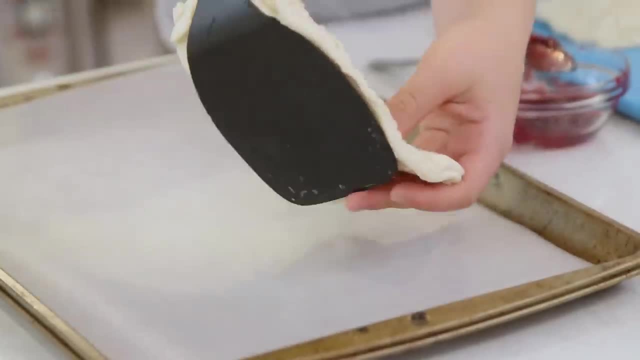 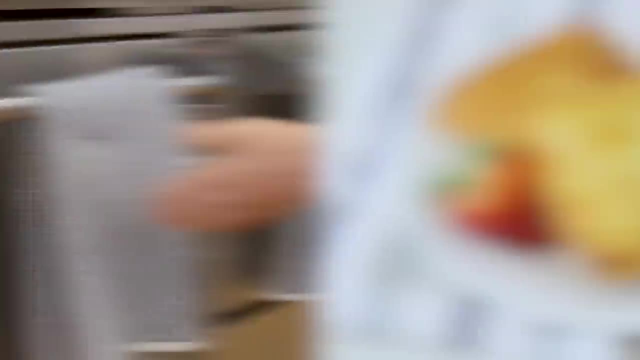 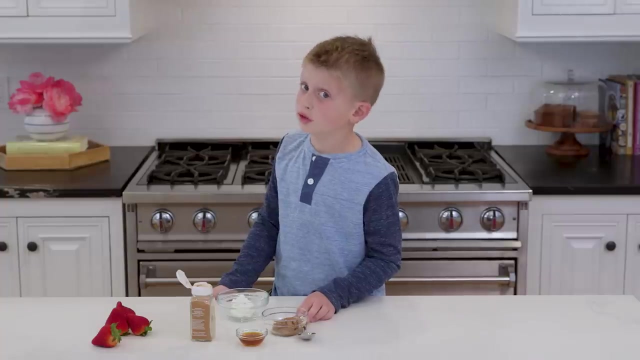 use a spatula to put them on a parchment lined baking sheet. Now into a 425 degree oven for 8 to 10 minutes. These are golden brown and I can't wait to give them a try. Next up, we're making fruit dip and I love good dip. I'm gonna dump my almond butter into my 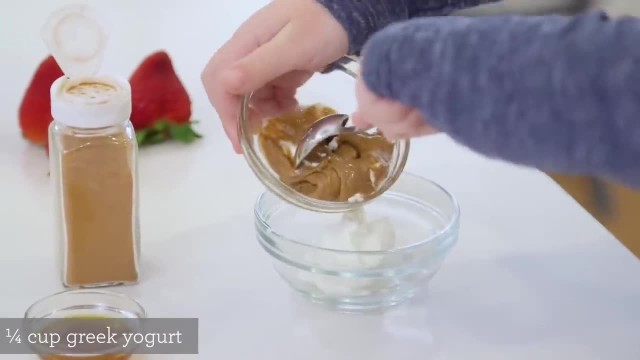 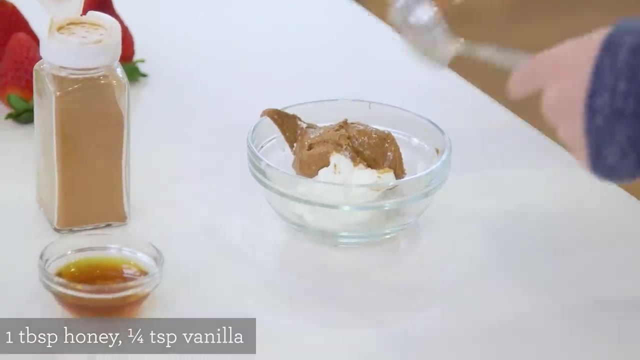 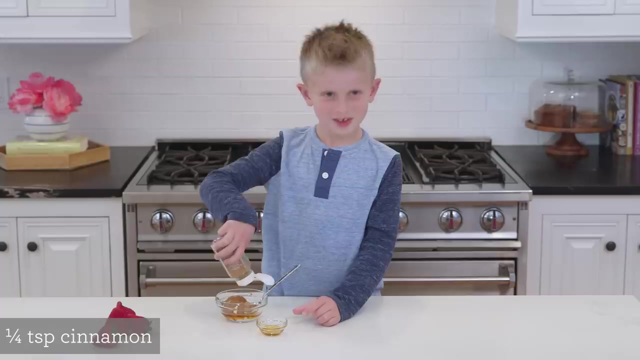 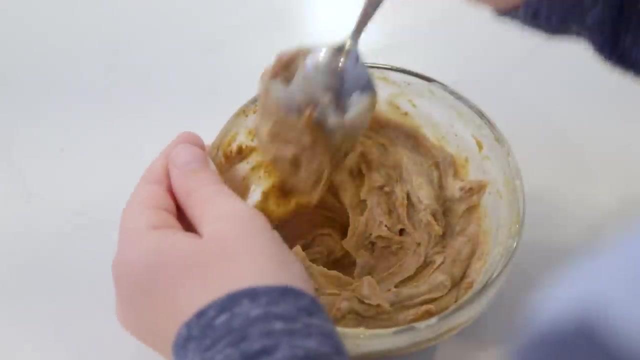 Greek yogurt. This stuff is sticky, but I got it all out. I have my honey and vanilla and I'm just gonna pour it in and then I'm gonna sprinkle some cinnamon and give it a squirt. Oopsies, Make sure you use two hands to stir. This goes good. All lets left is to dip our fruit Now. lets draw this today. 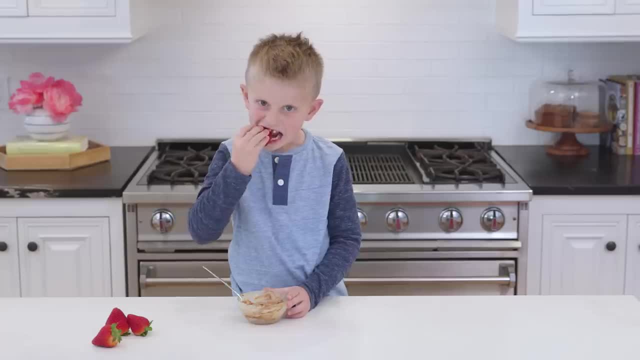 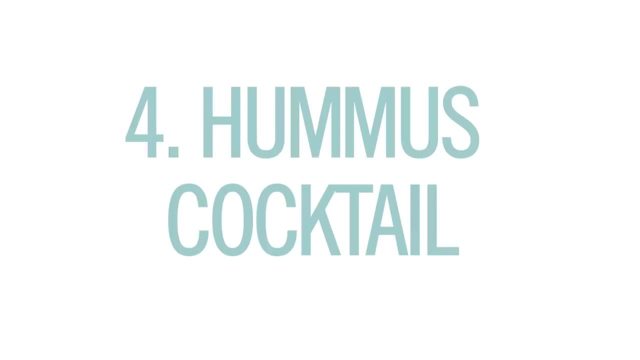 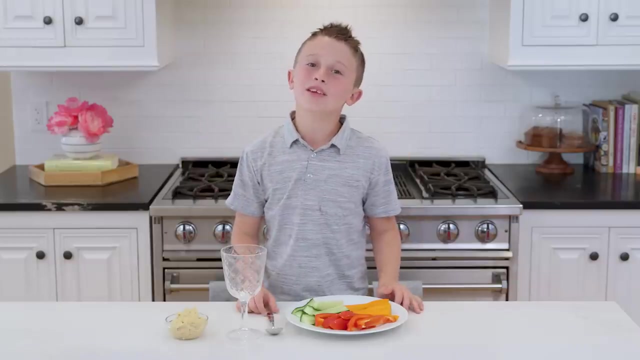 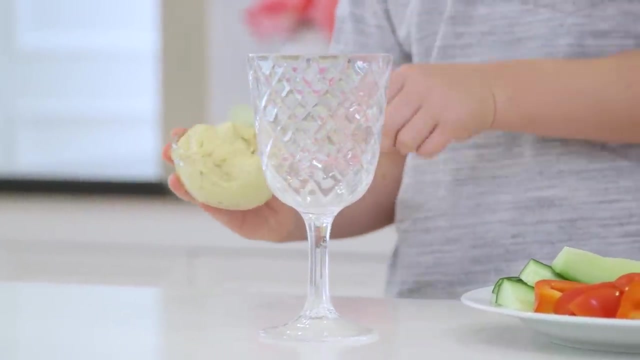 Mmm, this is good. Next up, we're making a hummus cocktail. Now, I'm not sure I would call homework time happy hour, but with this hummus cocktail it's pretty close. So. So we got some hummus right here and I'm going to scoop it into a plastic cocktail cup. 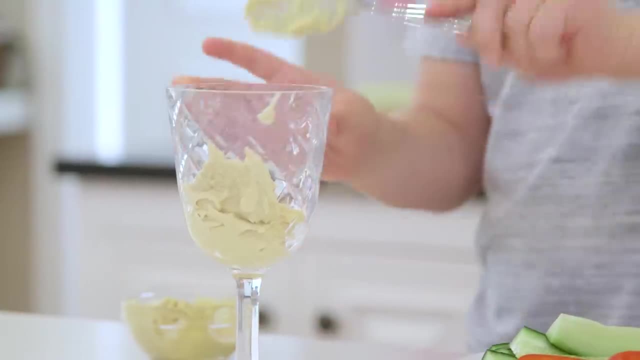 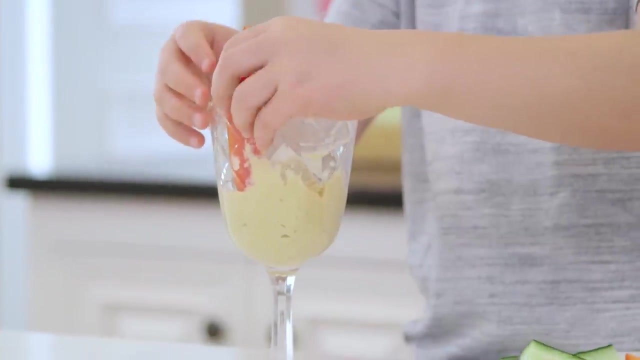 I'm trying not to let it get in the side of the glass Next up. let's do our veggies. So I've got a bell pepper right here. I like how they curve, So I'm going to put those on the outside to make sure they curve towards the inside. 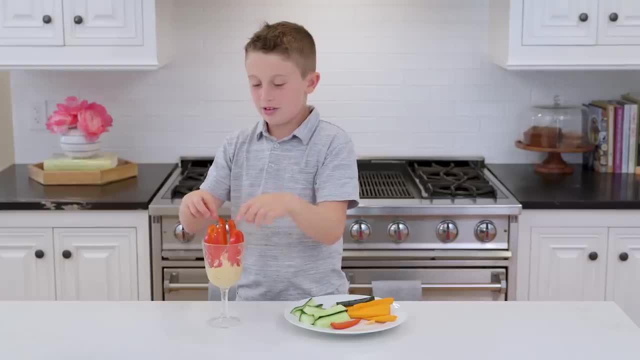 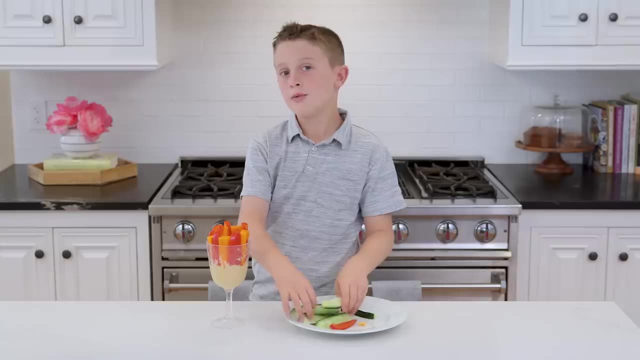 I like the bright red color. Mom says I don't have to use all of them, but I love my veggies, So now I'm putting some carrots in And finally we need some green in here, so we're going with cucumbers. 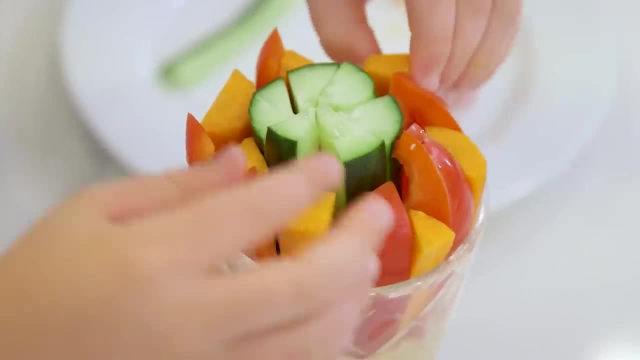 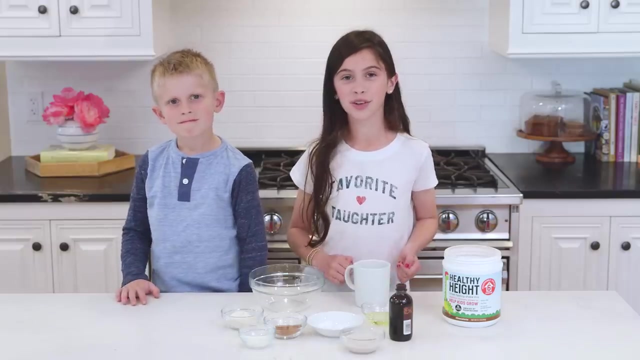 This is one way to eat your veggies. All right, this looks pretty awesome. cheers. And finally, we have mug cake. If you need something sweet to get you through that homework, this is it. We're even going to add some kid-friendly protein powder to power us through. 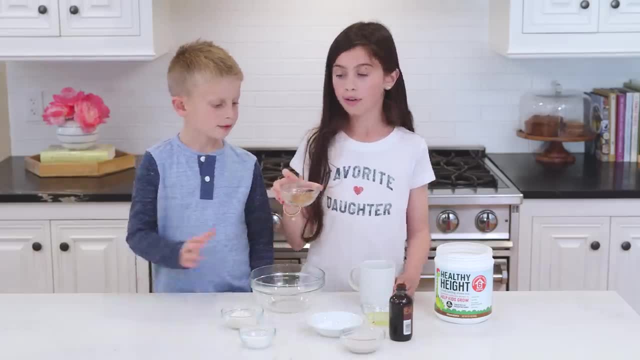 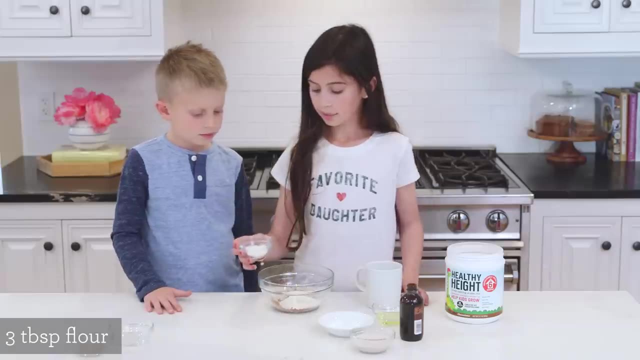 So let's go. First we're going to put in our cocoa powder, and next, Ryder, can you please put in that flour? Good job, Then I'm going to put in our sugar and then, Ryder, would you like to put in the baking?